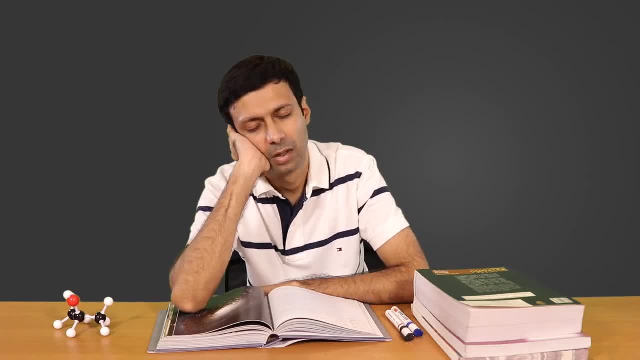 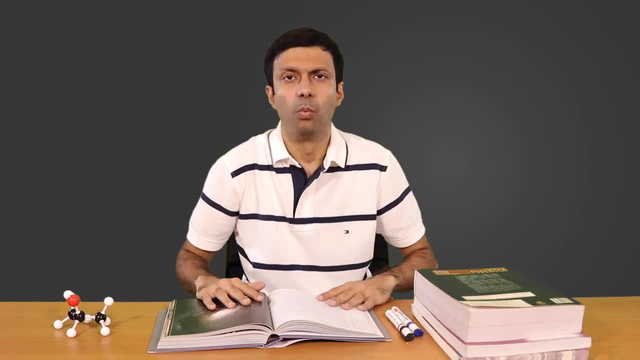 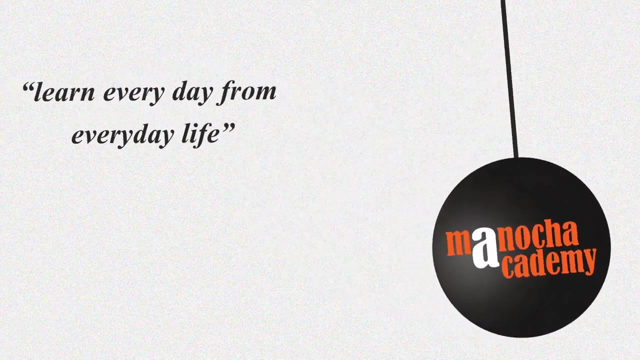 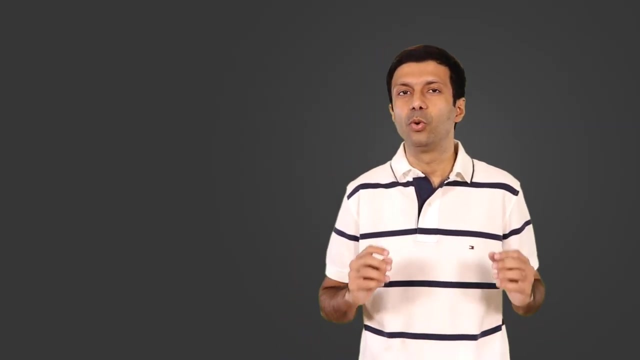 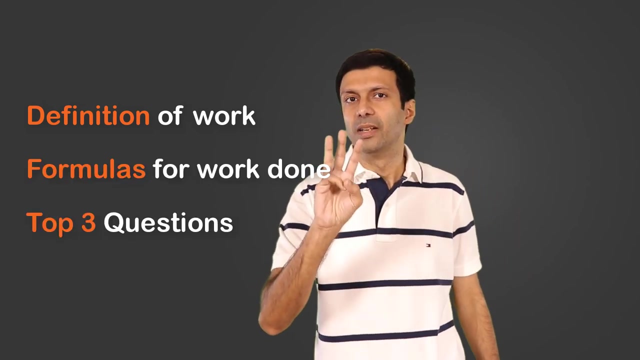 Don't disturb, I am very busy with work. What I need to make a video on work today. Alright, let's get started then. Hi friends, In this video we'll be doing the physics definition of work, the formulas to calculate work done, and then we'll do our top three test-oriented questions. 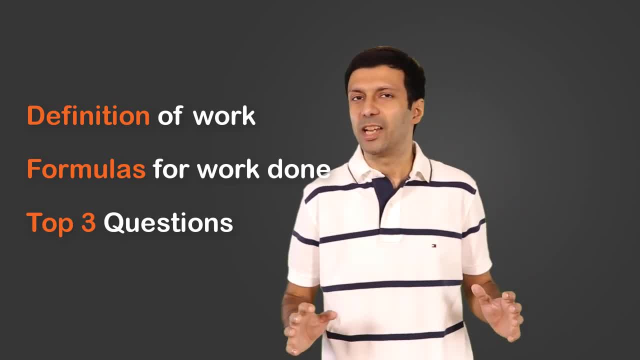 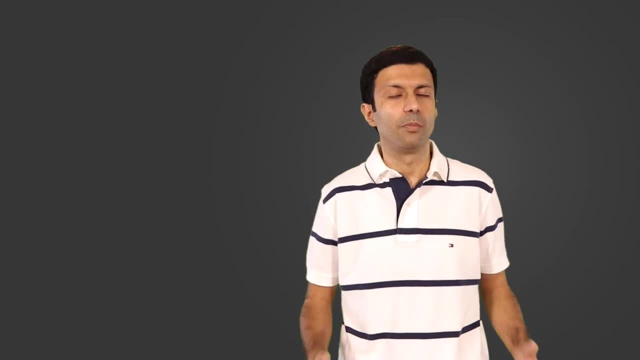 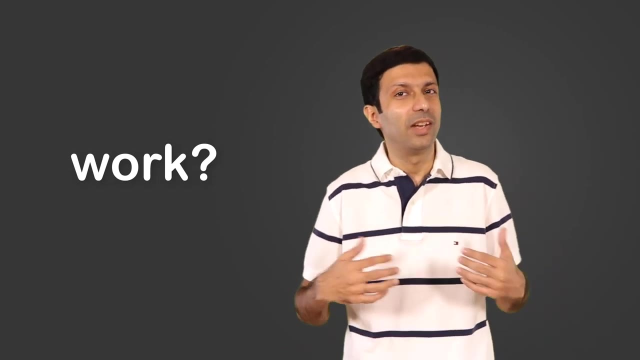 on this topic. I am sure by the end of this video, the concept of work will be really clear to you. Now, what comes to your mind when you hear the word work? Are you thinking about your homework or the work of cleaning up your room? For me, my work today is to make this video. 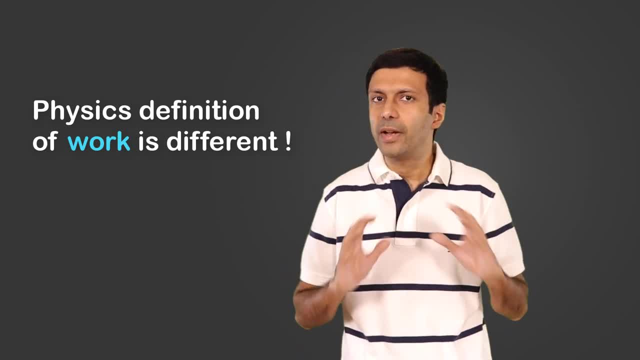 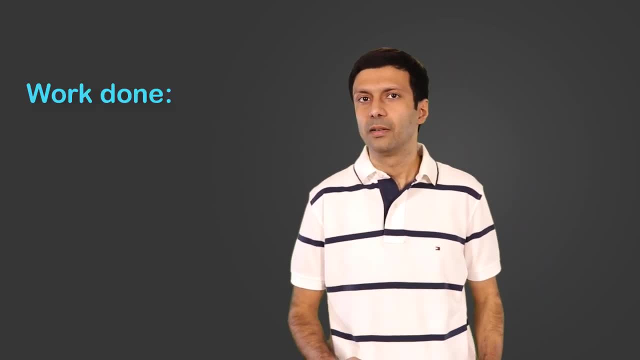 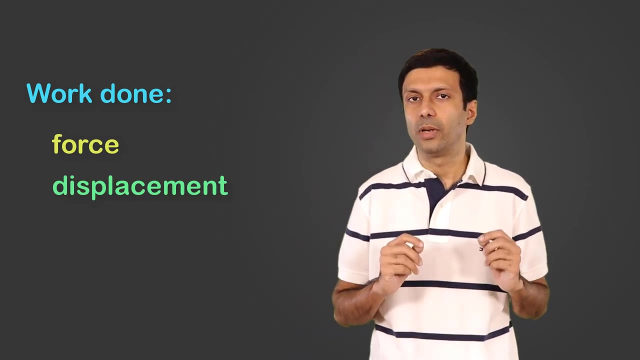 for you. The physics definition of work is very different from our everyday use of the term work. In physics, work is done when there is a force and there is a displacement involved. The formula to calculate work done is force into displacement in the direction of the. 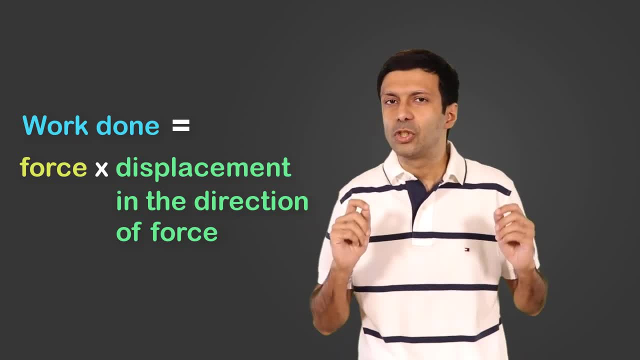 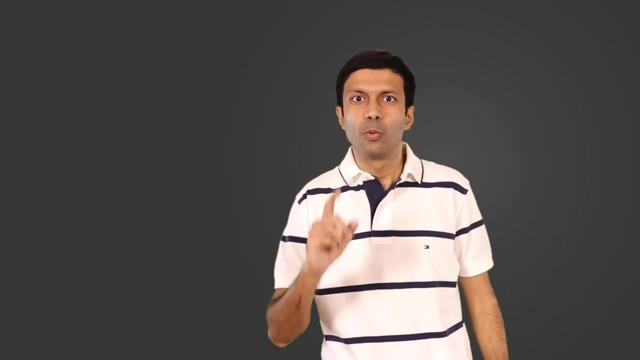 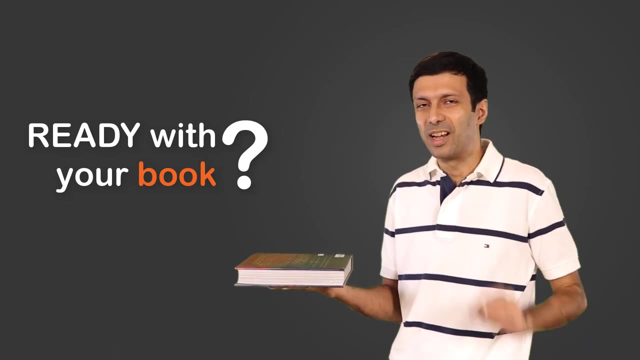 force To understand this. let's do a simple experiment together. For that I need you to get an object like a book. So pause the video right here and go and get a book. So are you ready with your book? I am ready with mine, Otherwise, 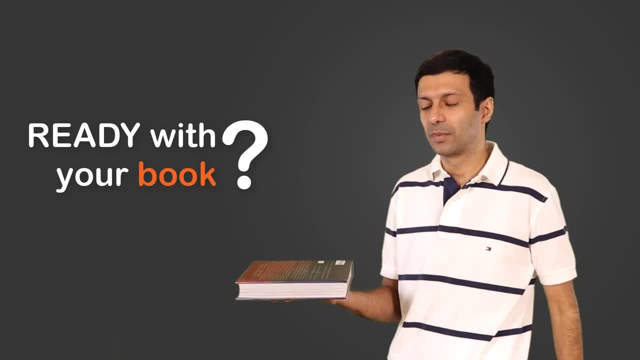 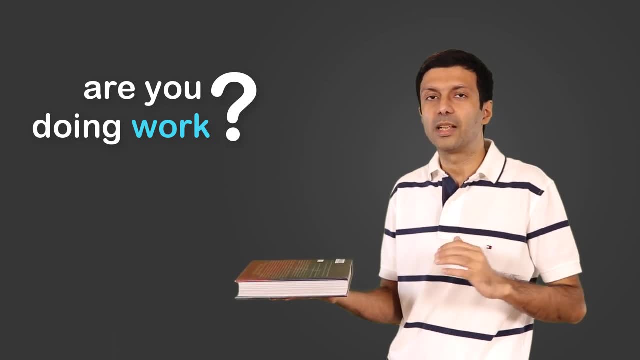 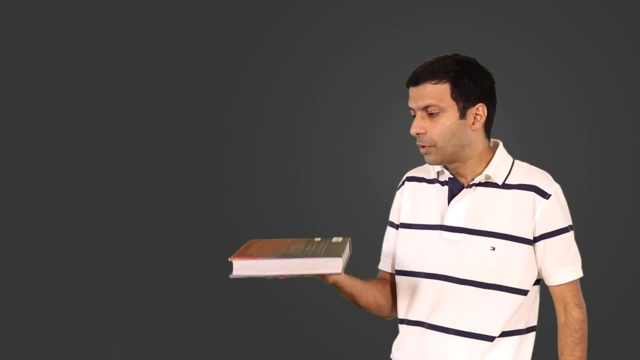 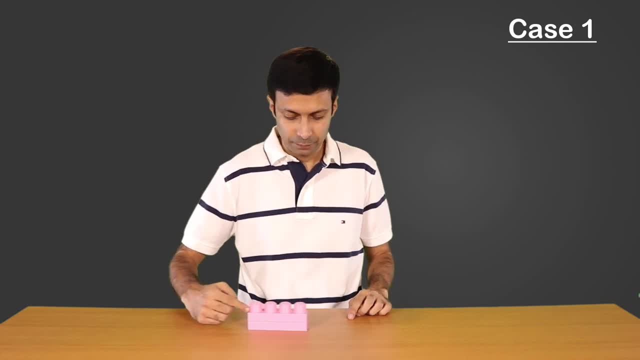 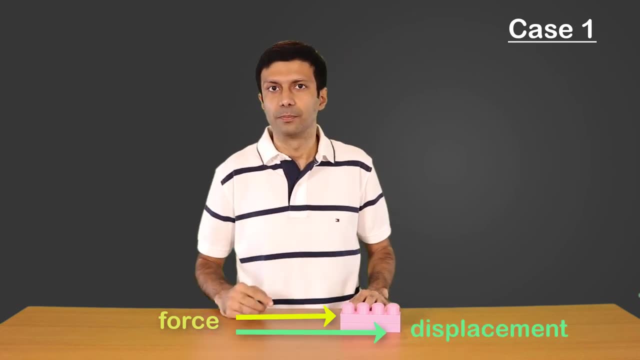 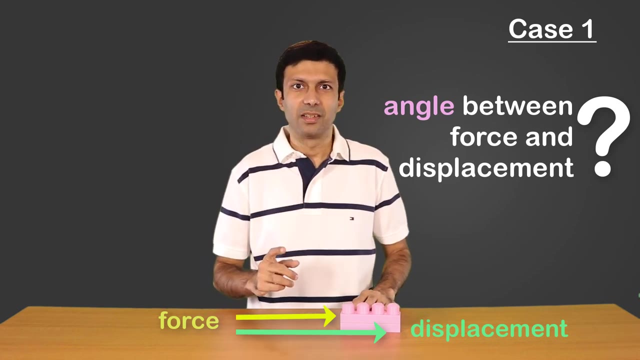 So when I push this block along the table like this, So when I push this block along the table like this, are along the same direction. So what is the angle between the force and the displacement here? That's right, it's zero degrees. 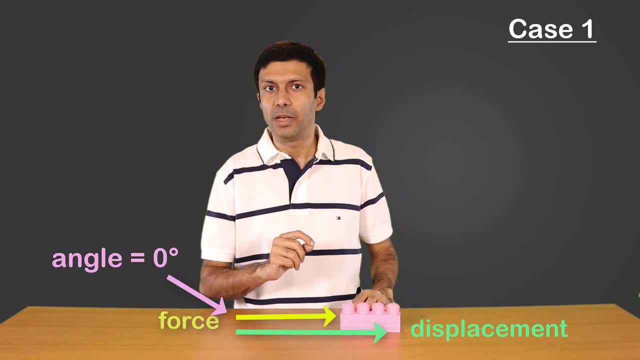 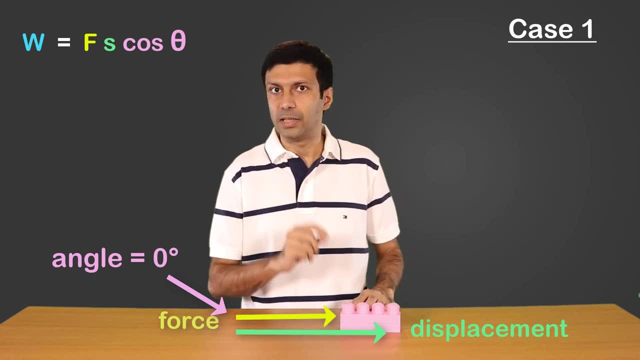 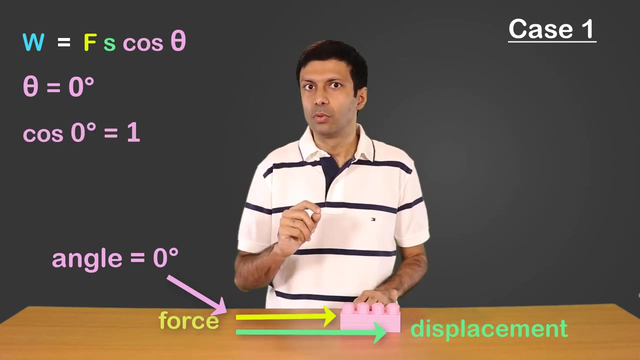 So if we use our general formula, our work done will be W equal to Fs cos and we'll consider it in the final product. So if we use our general formula, the final product, the final product know that the angle theta is 0 here and cos 0 is 1, so we get W equal to F into S. 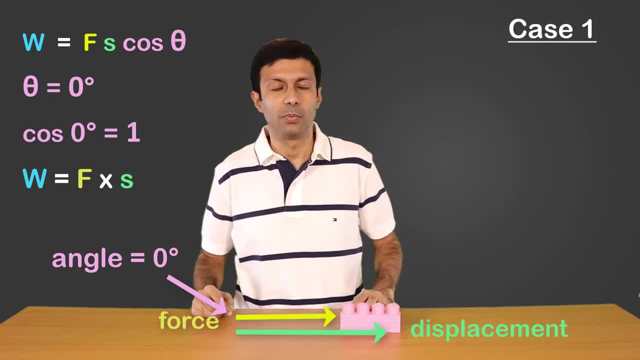 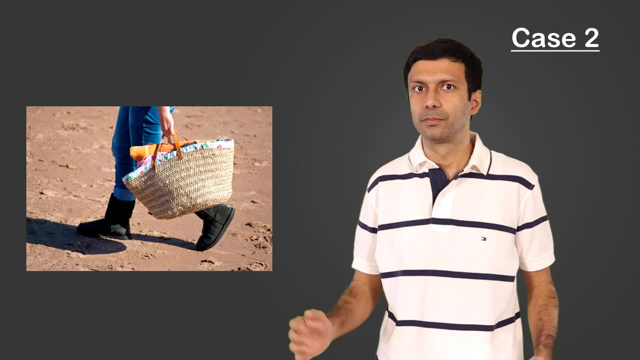 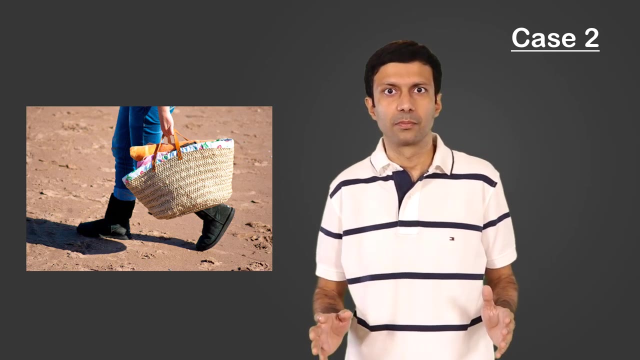 which is basically the first formula that we did in this video. case 2: suppose a person is walking carrying a bag, as shown in the picture here. so to find the work done we need to look at the force and the displacement here. so what is the direction of the force? so, since he is holding the bag, the force is in the 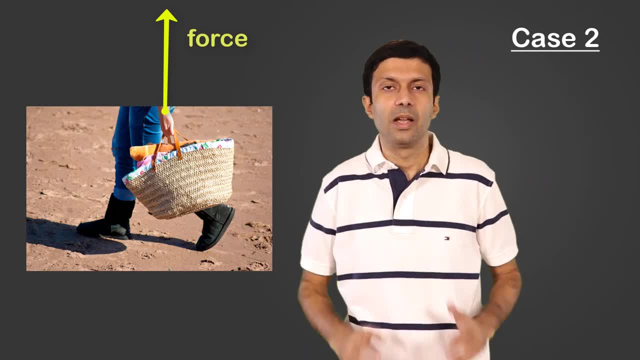 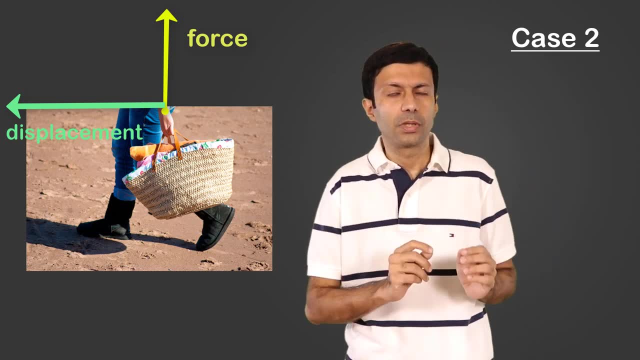 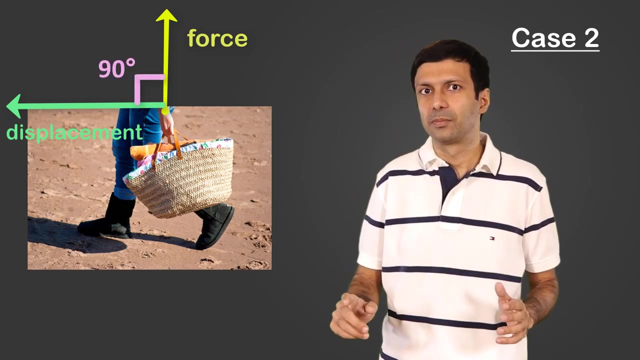 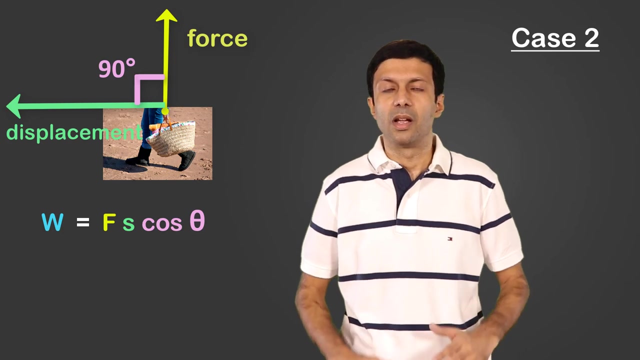 vertically upward direction and the displacement is along the path he is traveling. now what is the angle between the force and the displacement here? that's right, the angle is 90 degrees. so now let's use our formula: W equal to F, s, cos, theta, and we know that. 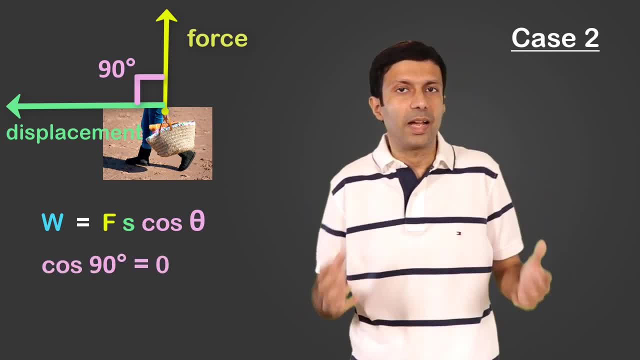 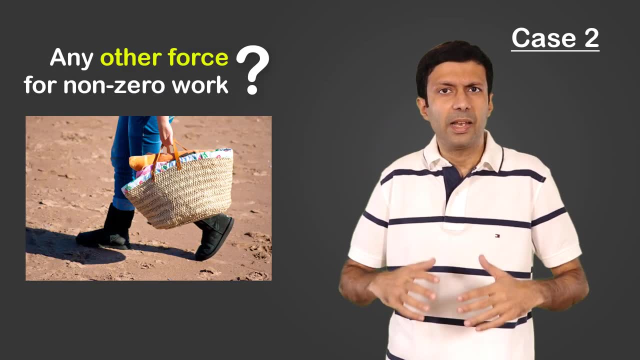 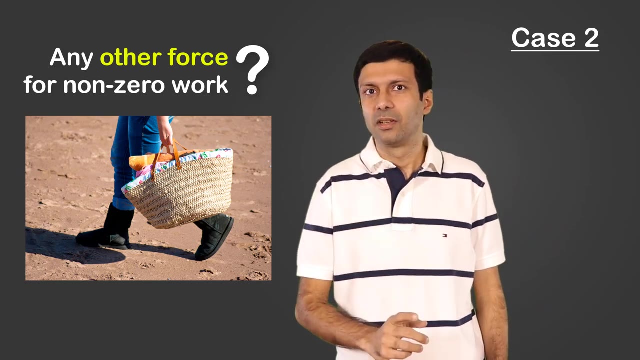 cos 90 is zero, So the work done actually turns out to be zero in this case. Now how is that possible? Is there any other force for which he's doing non-zero work? The answer is yes, It's the force of friction. So when he's walking along the path, he's doing non-zero. 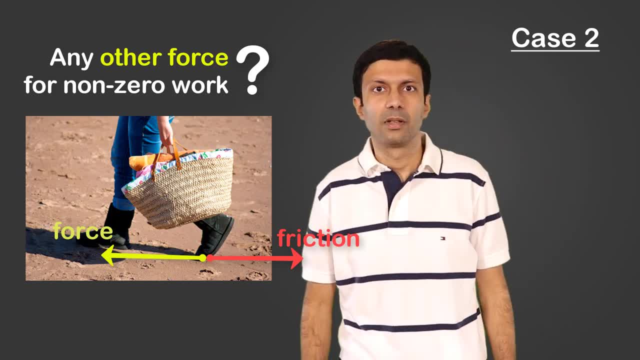 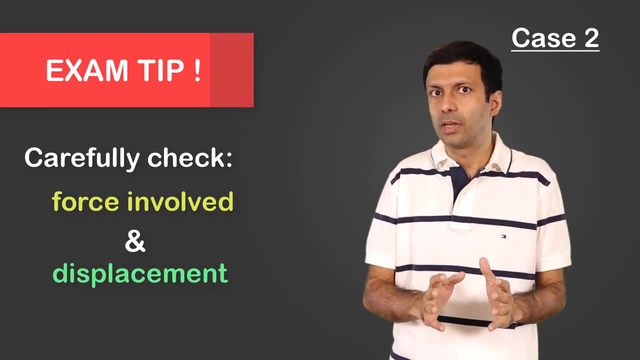 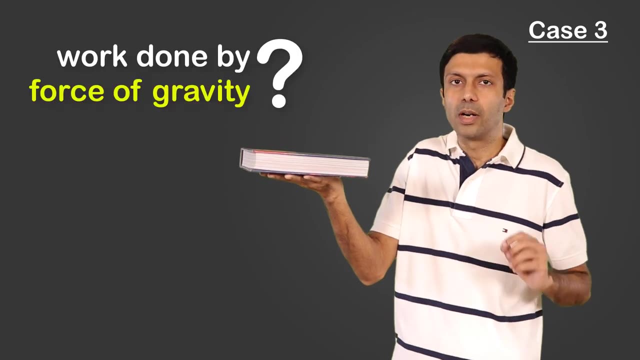 work against the force of friction. So an important exam tip is that to find the work done you need to carefully consider the force involved and the displacement Case 3.. If I lift the book like this, what is the work done by the force of gravity here? So, last, 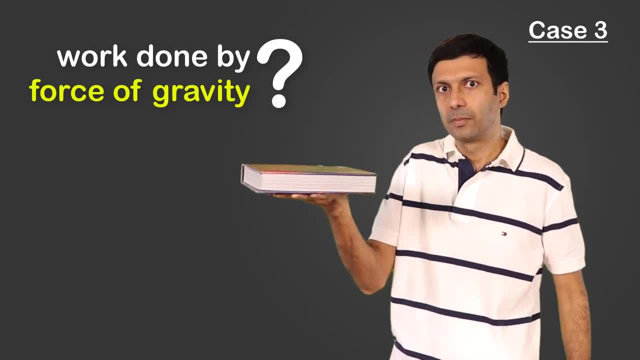 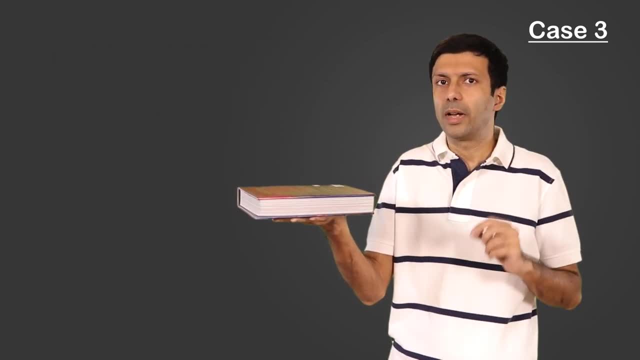 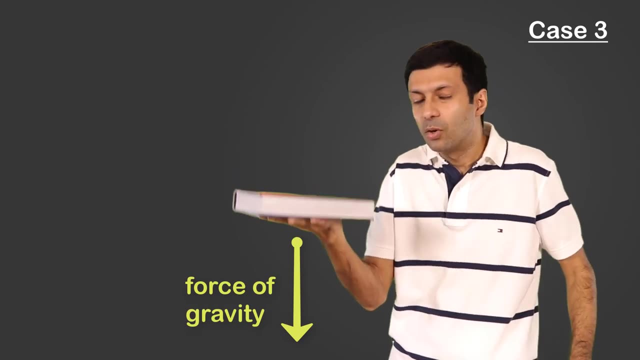 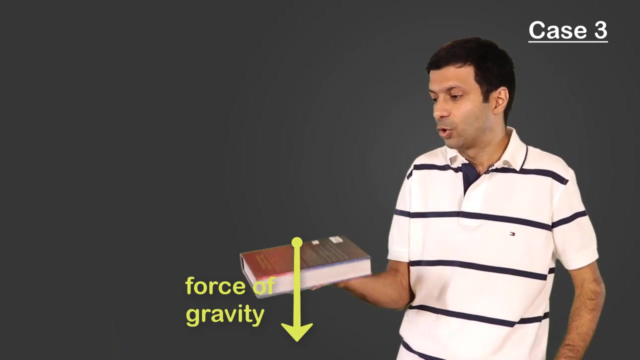 time we looked at what is the work done by us, But now we are interested in the work done by the force of gravity. So what is the direction of the force of gravity? That's right, It's vertically downwards, since it's the weight of the book. But what was the direction of the displacement here? 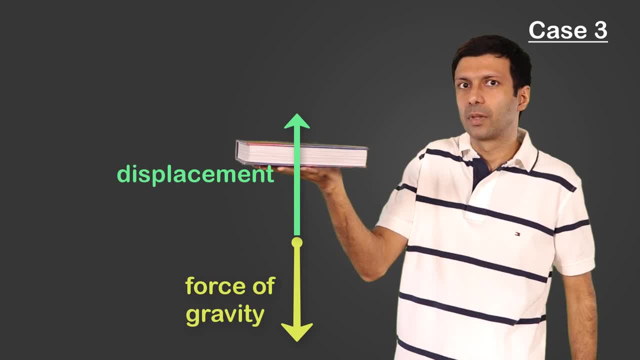 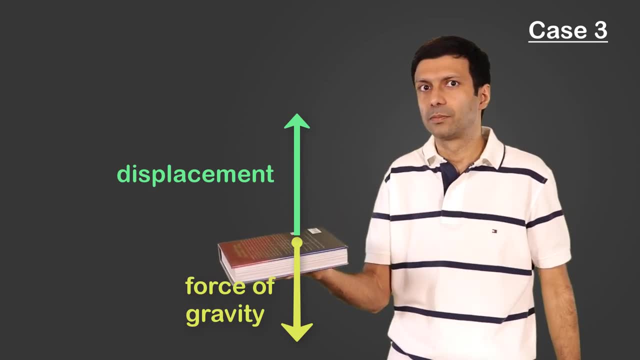 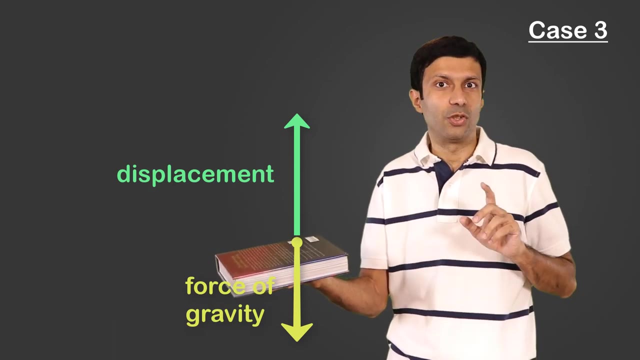 As you saw, it's vertically upwards, So the force of gravity and the displacement here are in opposite directions. So what is the angle between the force and the weight of the book? So the force of gravity and the displacement? It's not zero degrees, It's going to be 180 degrees here. So now,